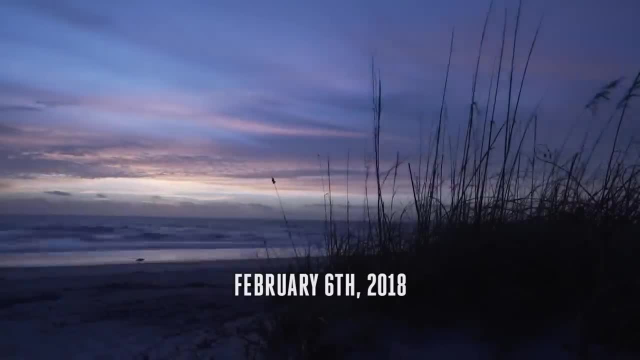 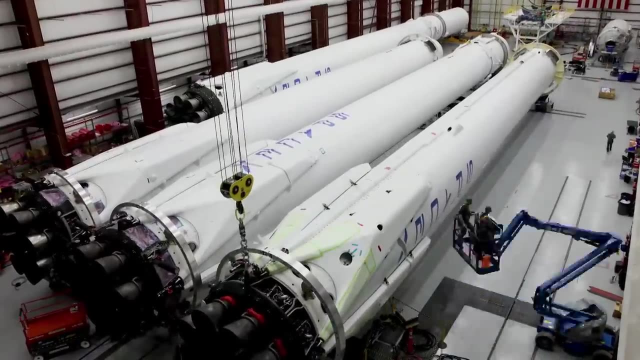 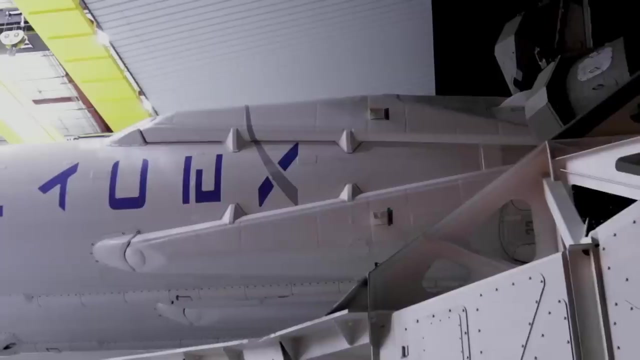 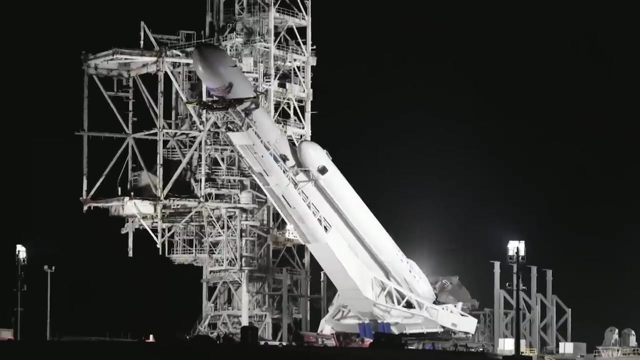 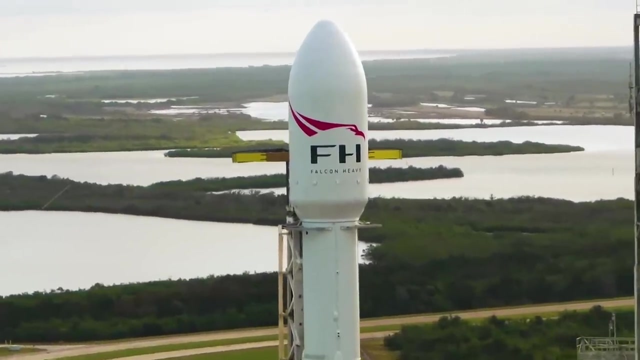 Most space organizations- government or commercial- have set their sights too low. They've really gotten built relatively small rockets, And Falcon Heavy is the first time that there's something that's arguably even in the super heavy class or somewhere between heavy and super heavy. 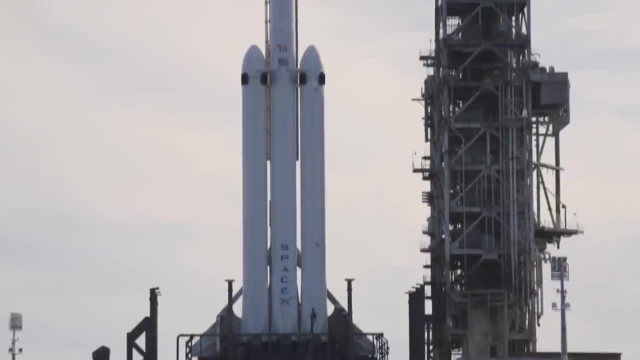 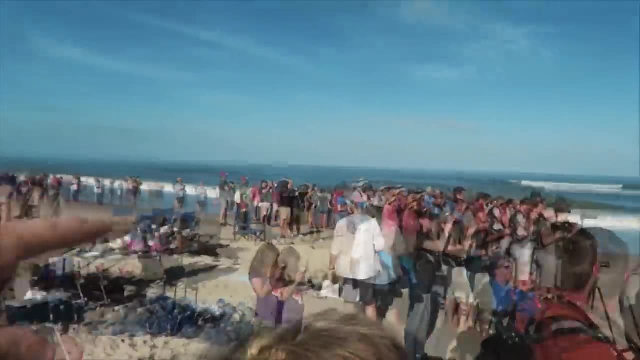 You know, 5 million pounds of thrust is a really crazy amount of power, More than twice as much payload as any other rocket in the world. It can launch things direct to Pluto. No stop needed. Hotels in the area are completely sold out. Working lots are packed. 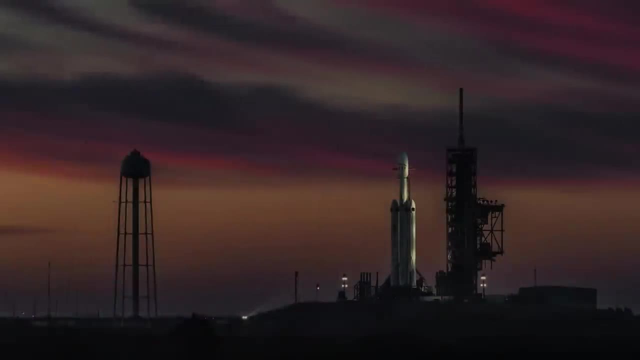 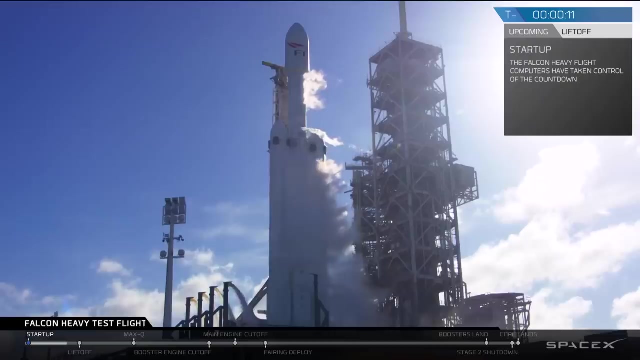 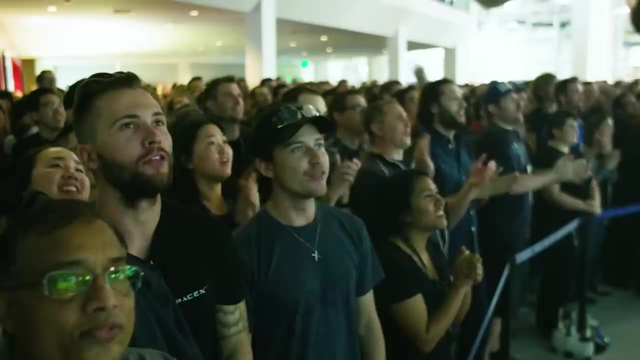 It's like the first time something exciting has happened in rocket launch in a very long time. Falcon Heavy is configured for flight T-minus 15, stand by for terminal. count SpaceX Falcon Heavy go for launch 10, 9,, 8,, 7,, 6,, 5,, 4,, 3, 2, 1.. 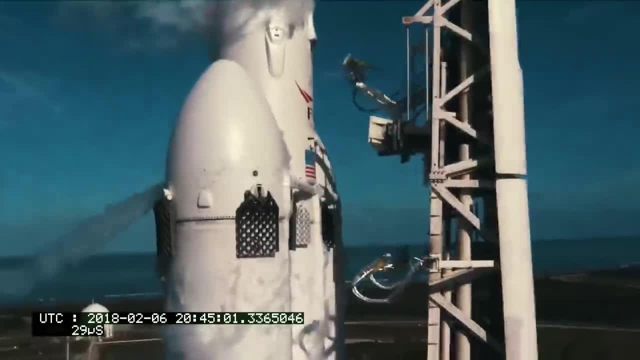 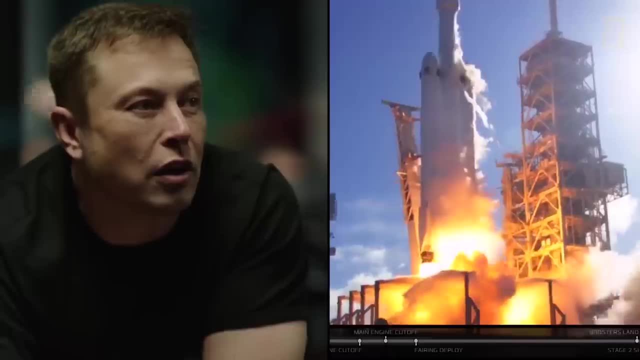 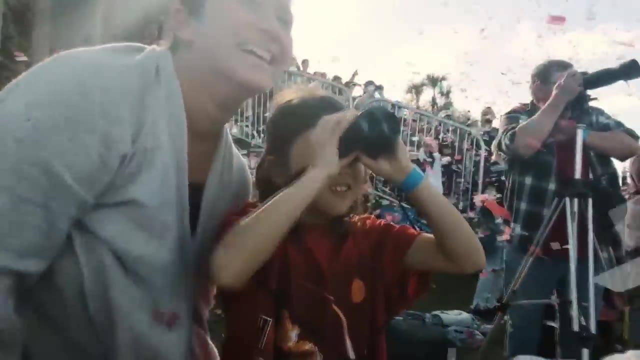 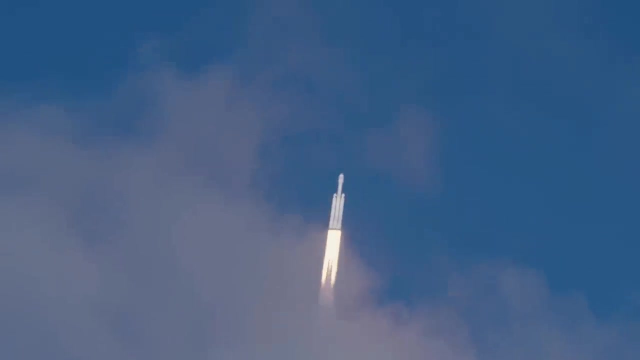 It's on. It's on Falcon Heavy. Falcon Heavy heading for space on our test flight, Building on the history of Saturn 5, Apollo Returning 10-30-9-8, an interplanetary mission Vehicle is supersonic. 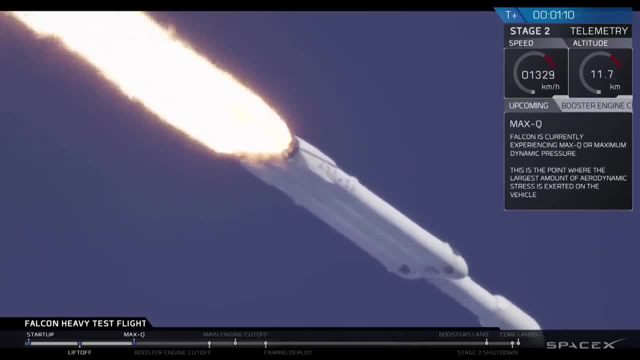 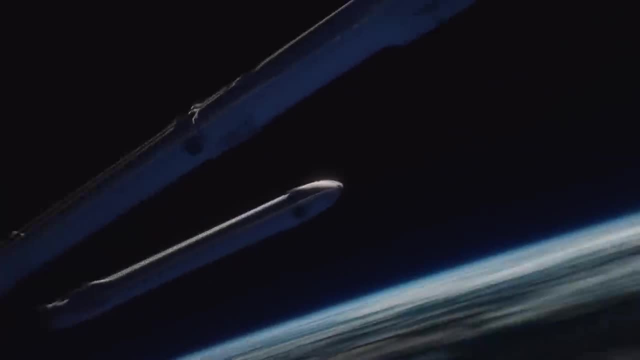 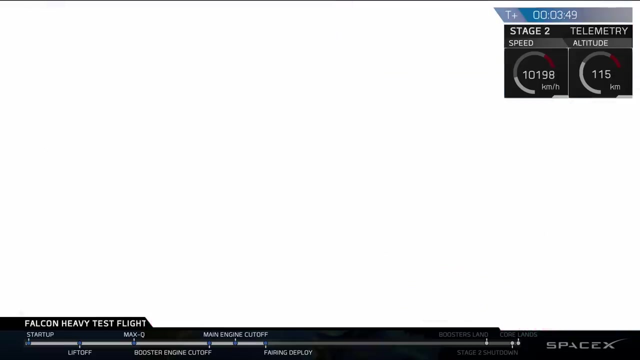 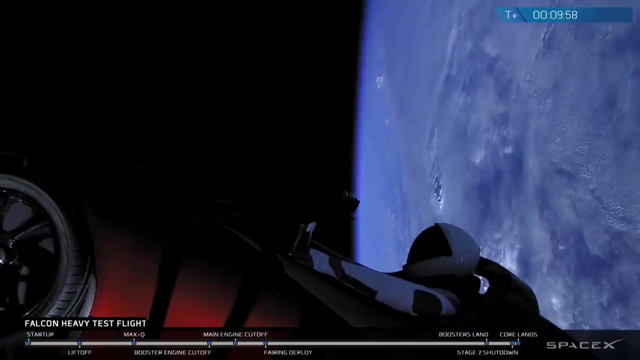 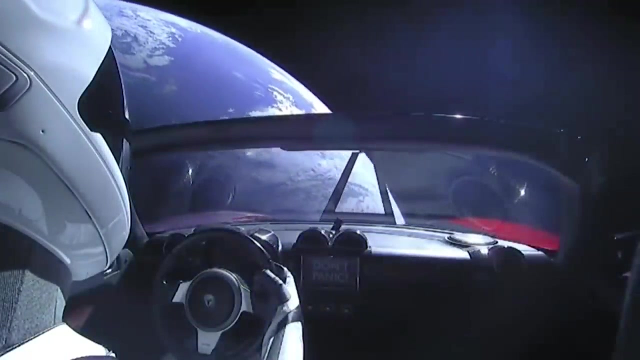 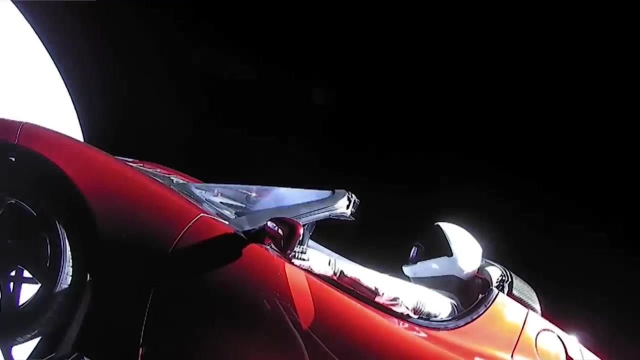 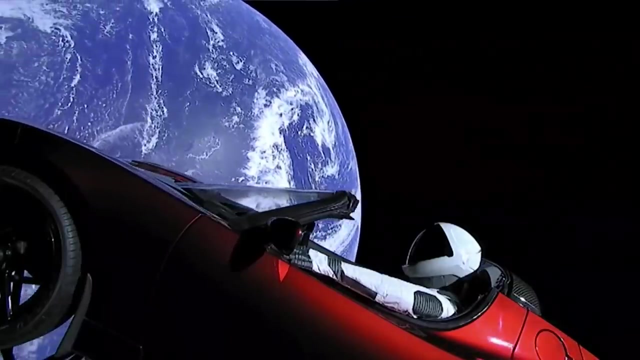 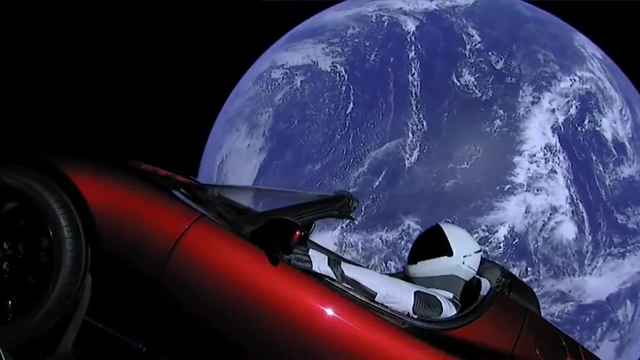 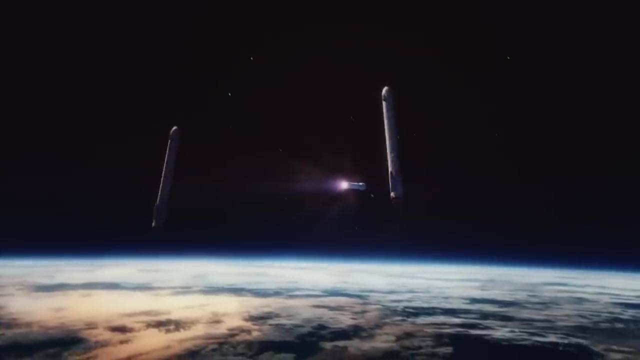 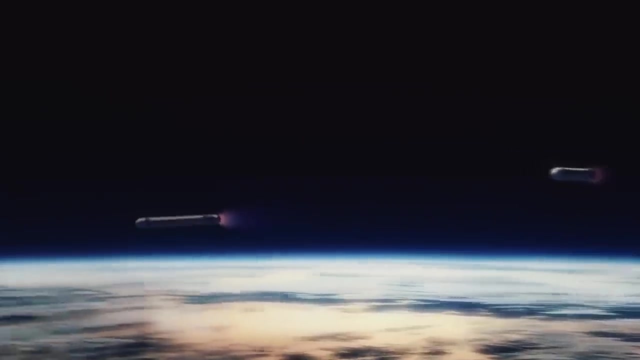 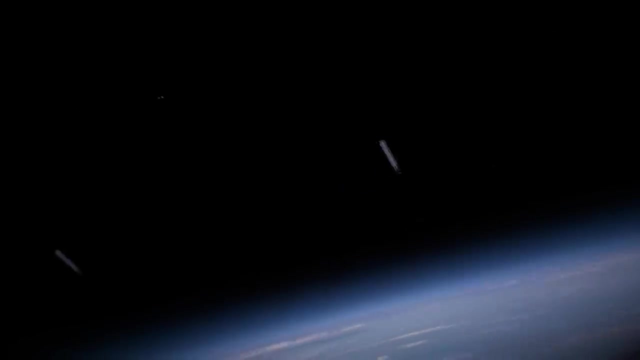 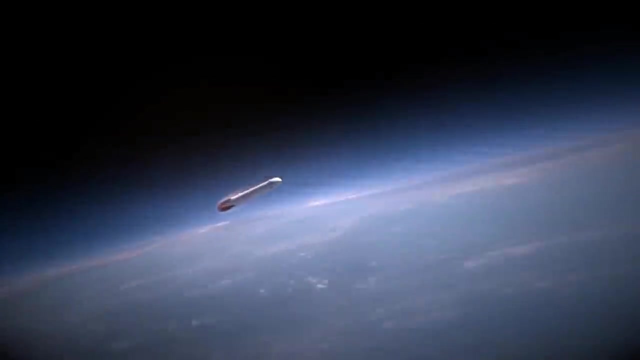 You heard the call out Vehicle is supersonic Saturn, shut down Side boosters Vehicle. We find he's landing. We have environmental vaccin s mess parts. Besant, Let's fly, Let's fly. f They're headed towards Earth and they're about to begin their landing burns. 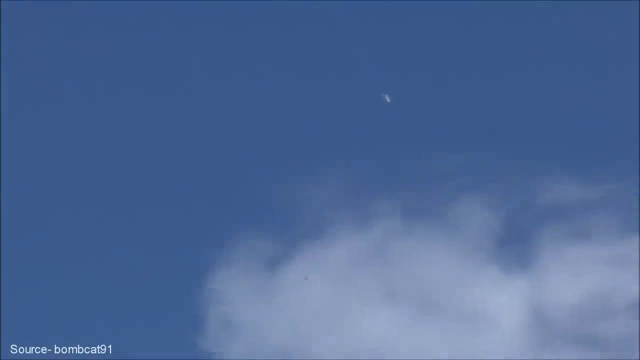 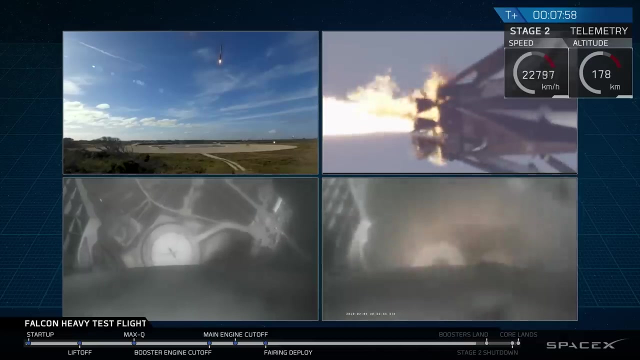 And that landing burn has started. They're seriously going to be on track towards their respective landing zones. Landing zones: landing lights have started on the plane. Starbazer's landing lights have deployed. Gotcha, I see it. Yeah, I got him. 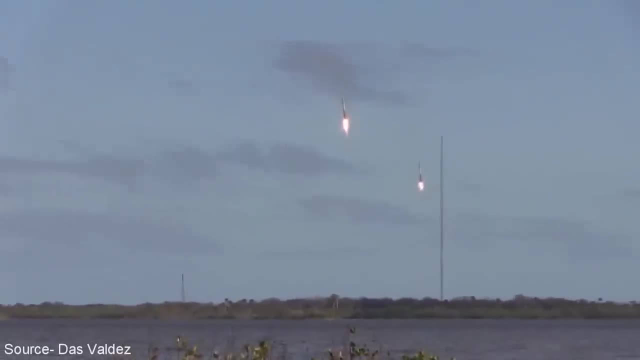 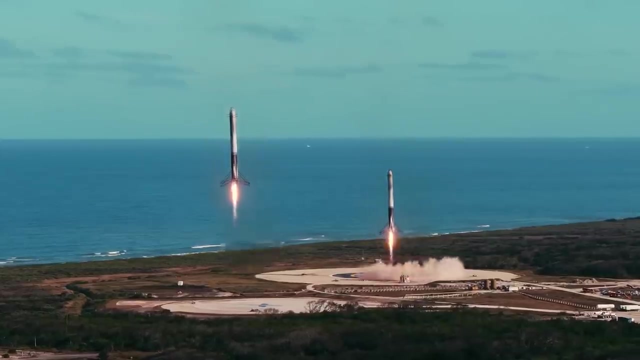 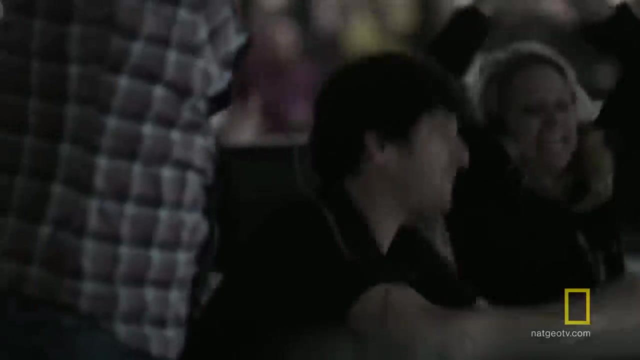 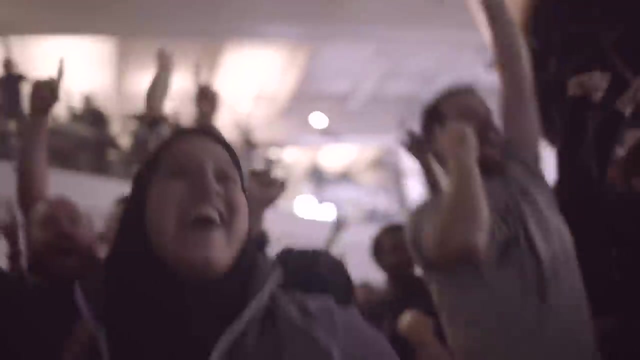 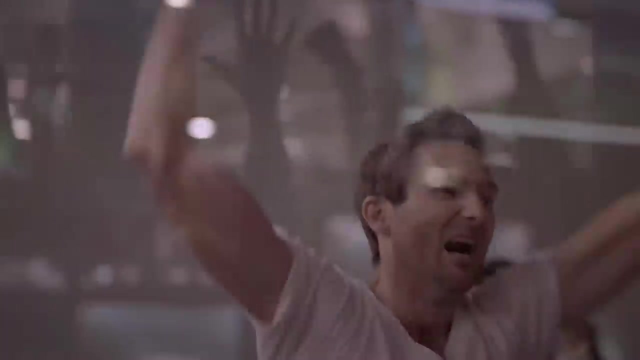 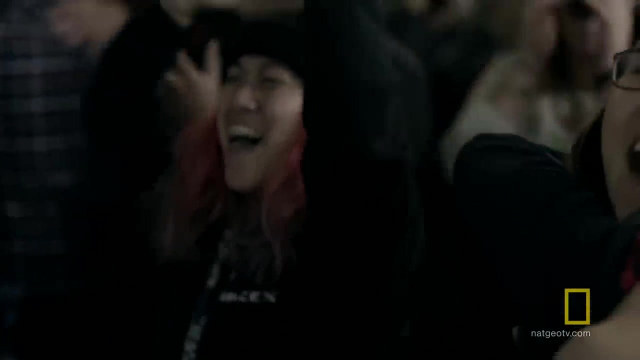 They're there, y'all. You've got to be kidding me. What? What is this? And the Falcons have landed '". Oh no, What's happening? I know this is did not come from Bob's left arm until me. 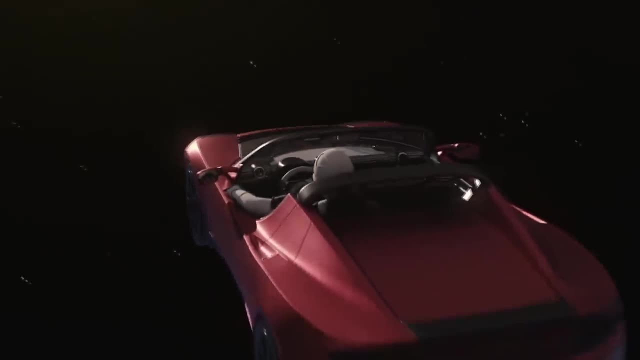 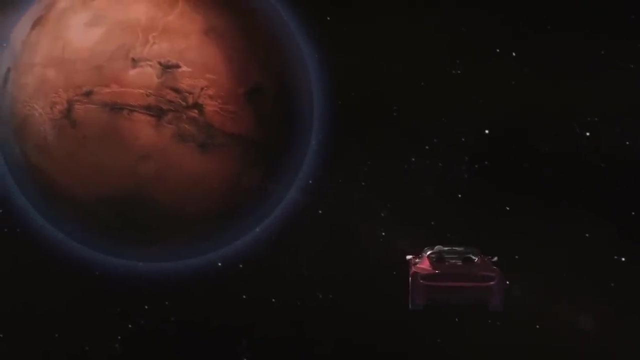 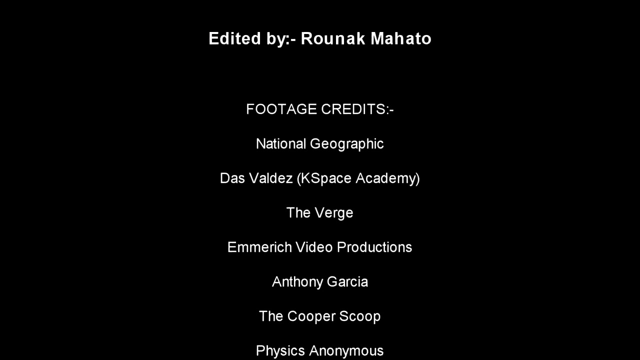 I thought she was right and thought it wasn't What. I'm sure one more did come from the other side of her arm. Maybe she just has to leavearla, I can't tell. Is that the whole thing? Thanks for watching.